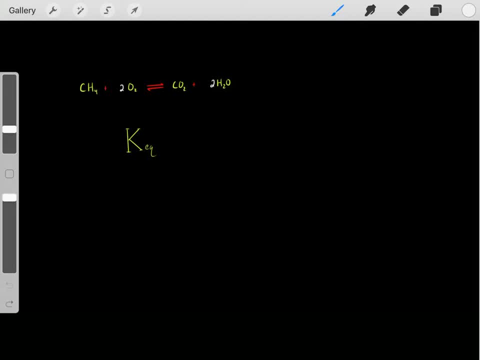 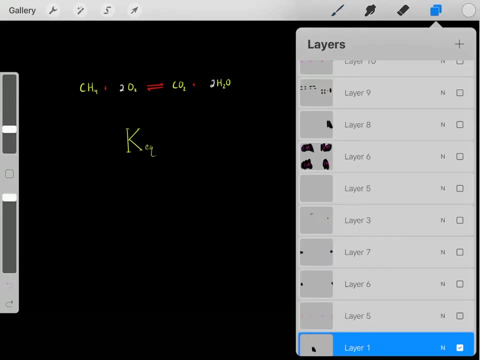 the reaction at equilibrium. So what do I mean? Well, let's take this reaction and let's determine what its equilibrium constant is. How do we determine this reaction's equilibrium constant? Well, first we just have to have any random concentrations, just any original conditions. 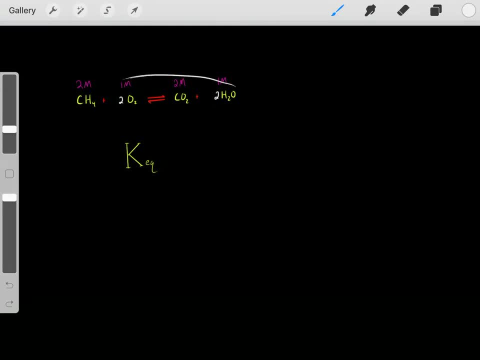 It doesn't matter what these initial conditions are. We just have to have conditions and we need to let this reaction react. We know it's going to react With these initial concentrations. this reaction is going to react And as it reacts, these concentrations are going to change. 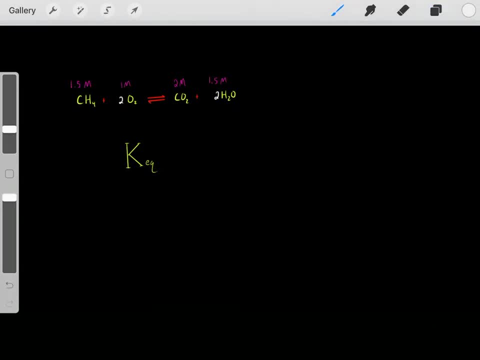 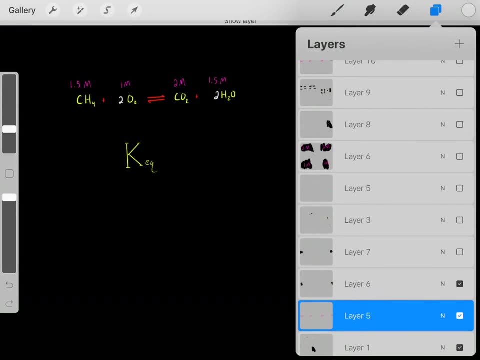 So, as it reacts, the concentrations are going to change. And don't worry about the stoichiometry and specifically how the reactions change. The point is, we have these initial conditions, then it's going to react. As it reacts, the concentrations will change. 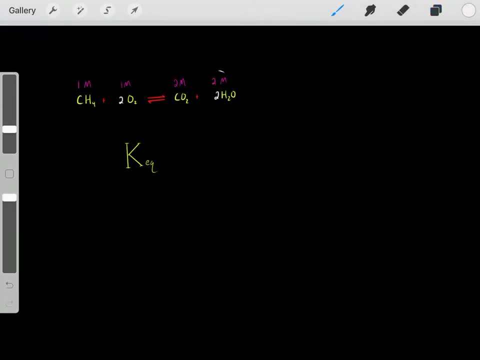 Then eventually we'll reach an equilibrium. Eventually we'll reach equilibrium concentrations And we know we're at equilibrium because the concentrations aren't changing. We've reached an equilibrium state where the concentrations aren't changed, so we're at equilibrium. So, now that we're at equilibrium and we know the concentrations at equilibrium, 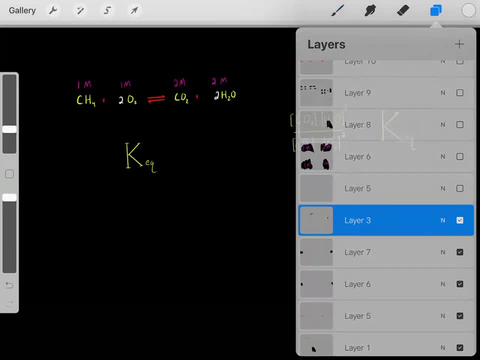 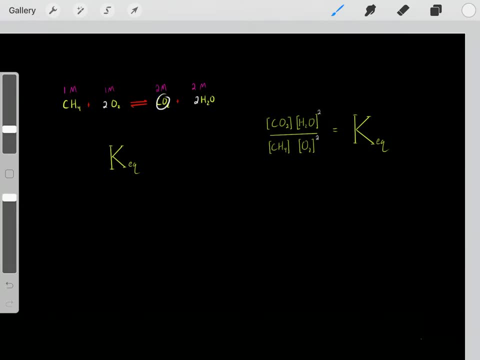 now we can determine the equilibrium constant using this simple equation, And it looks complicating. What's going on? It's actually not so bad. Essentially, what you do is you take the concentration of these products. Remember, these are the products and these are the reactants. 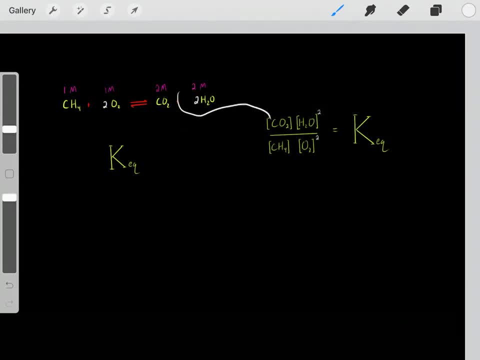 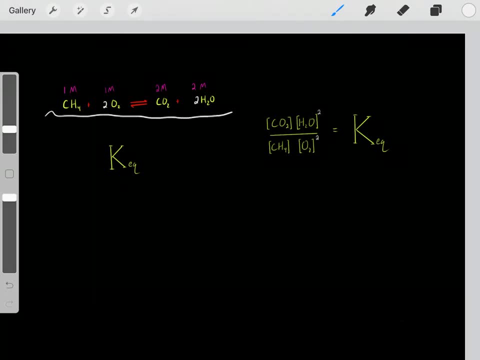 So you take the concentration of the products and put them in the numerator, Then you take the concentration of the reactants and put them in the denominator, And again, and something else is you need to see the balanced equation And you can't ignore the coefficients. For example, this water. 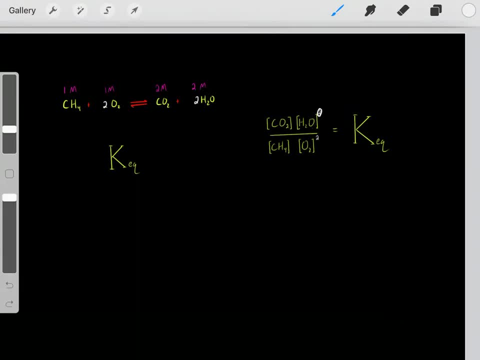 has a coefficient of 2.. So, therefore, this water concentration goes to the second power. And again, this oxygen has a coefficient of 2. So this oxygen concentration will go to the second power, And I know this looks complicating, but it's not so bad. You essentially take the concentration. 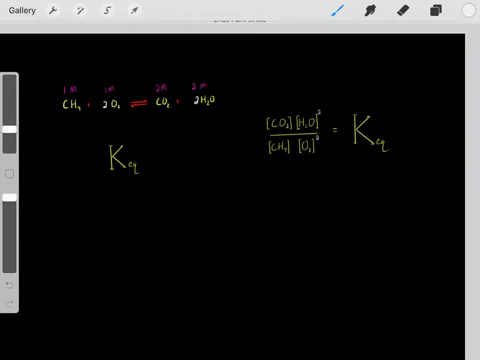 of the products. So this guy, this product, and then this product, and you put them in the numerator. then you take the concentration of the reactants and put them in the denominator, plug it in here, and plug this guy in here, And then again, don't forget these powers and put them to these powers. But again you just 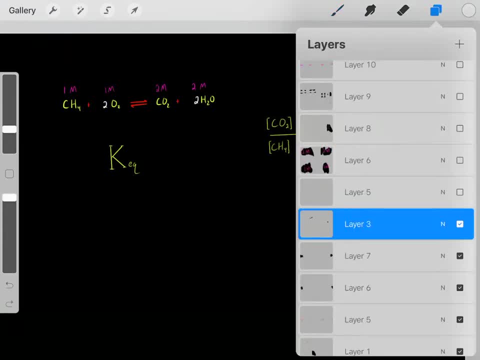 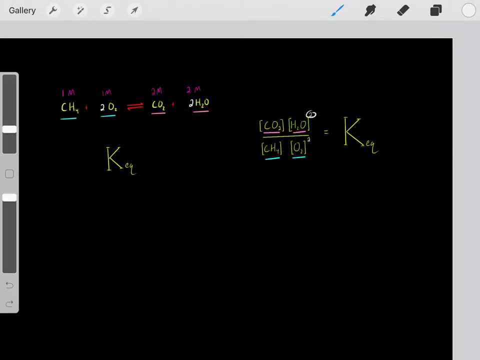 simply use this equation and plug it in and I'll tell you the equilibrium constant. So plugging in and again. so remember it's just the products over the reactants, And then again you multiply them and put them to the respective powers. So now, if we plugged in all these concentrations, 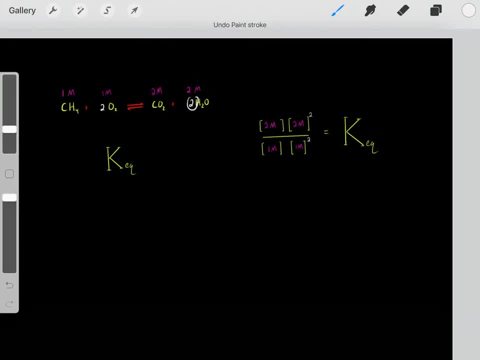 we this would. we would plug in two here, we plug in two here, And again it would go to the second power. Then again we'd plug in one here, put it to the second power, and again, et cetera. 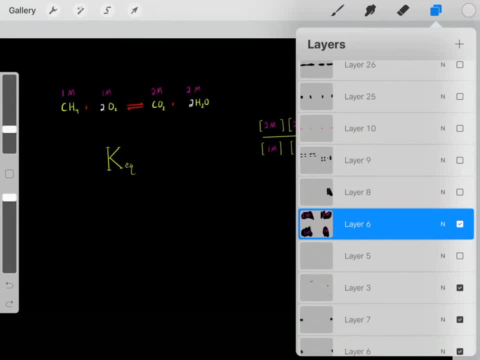 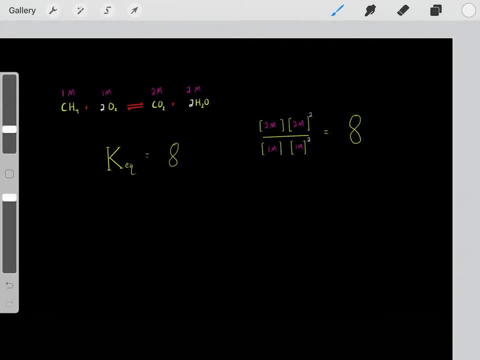 plug in one here and just multiply it And I'll give you the KQ. And if you did this, we'd get a KQ of eight of eight. So now we know this reaction has an equilibrium constant of eight and it's a. 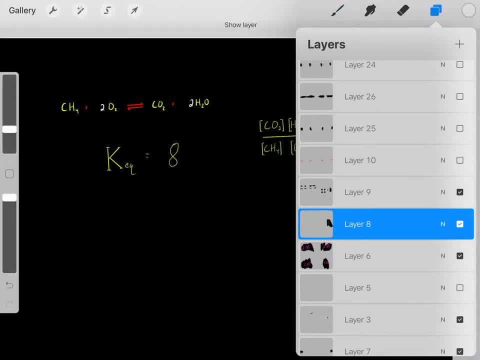 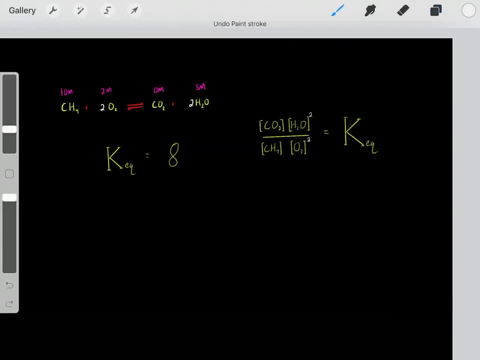 number that describes this reaction at equilibrium. And something important to realize is it doesn't matter what those initial concentrations were. For example, let's say we had these arbitrary initial concentrations where we had a large concentration of this guy, then two molar of this guy. Let's say we had none of this guy and five molar of this guy. 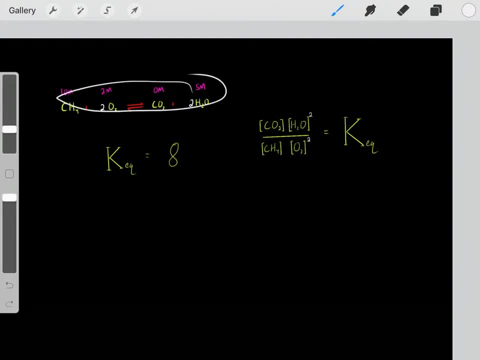 It doesn't matter what the initial concentrations are. We would let it react, It would react and eventually we'll reach equilibrium where we'll have certain concentrations at equilibrium. So if you plug in those concentrations, once we've reached equilibrium, into this equation, where again you would plug in this concentration here, this concentration here? 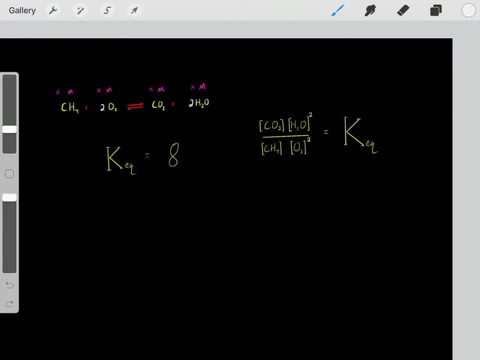 and et cetera, and put them to these respective powers and plug in those. So again we let it react, We reach equilibrium. We took those concentrations at equilibrium, plug them into this equation and it will always give eight, It'll always equal eight, because that's the equilibrium constant. It's a constant. This: 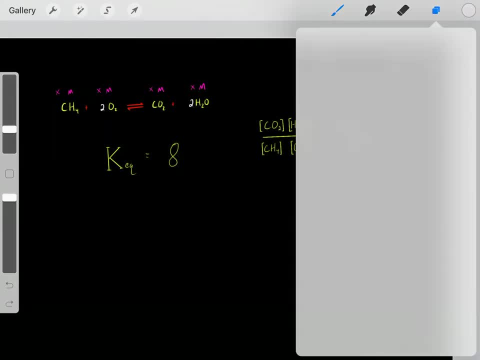 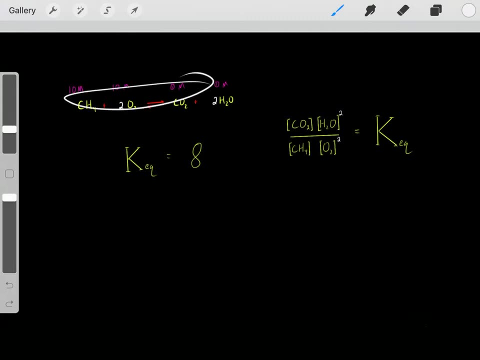 reaction has an equilibrium constant of eight. So again, it doesn't matter what the initial concentrations were. For example, we could have these crazy initial concentrations. We know it'll react. It'll react, Eventually it'll reach equilibrium concentrations And we plug in. 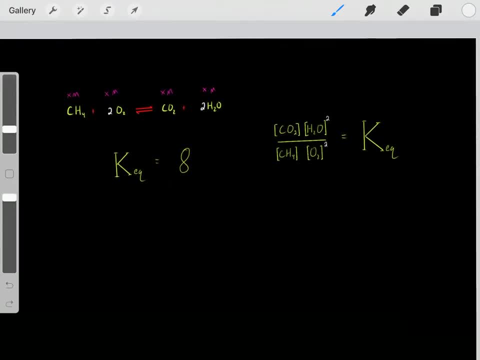 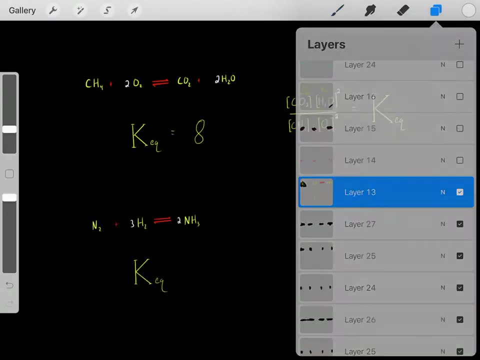 those equilibrium concentrations into this formula and it will always equal eight. So we know this is an equilibrium constant of eight. But let's do another example just to really illustrate what's going on. So let's say we have this chemical reaction. We know all chemical reactions have. 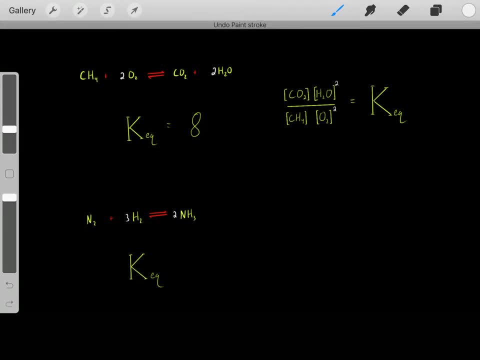 an equilibrium constant, which is just a number that describes the reaction at equilibrium. So how could we determine the equilibrium constant of this reaction? Well, again, we just have initial concentrations. It doesn't matter what they are. We have these initial concentrations and we let it. 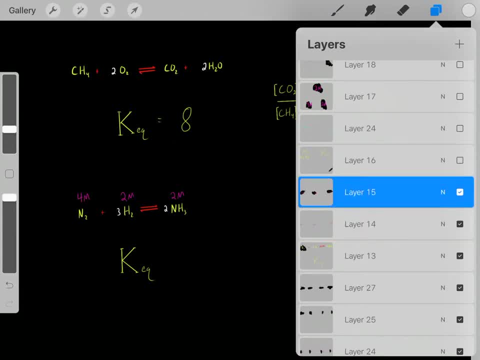 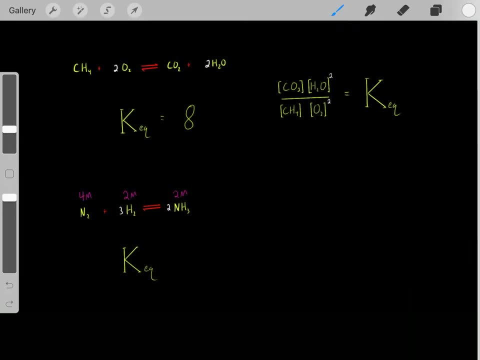 react. We let it react and eventually it'll reach an equilibrium. It'll reach equilibrium concentrations And again the stoichiometry and how it reacts. we know that it's an equilibrium. we reach these equilibrium constants. Don't really worry about it, Just know it reacts and 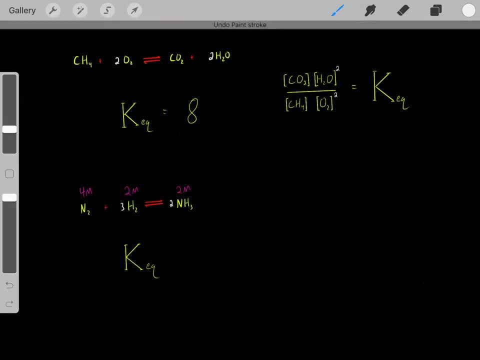 eventually we reach an equilibrium with these equilibrium concentrations. Now that we know these concentrations at equilibrium, we can plug it into our Keq equation. And again, remember, it's just the products in the numerator and the reactants in the denominator, And then again. 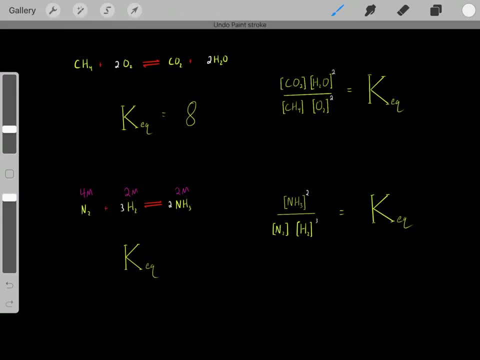 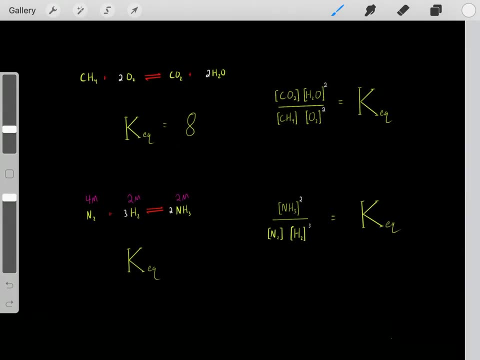 you also need to know the balanced equation with the coefficients. And again, this, because it's a coefficient of two, goes to the second power, And this, because it's a coefficient of three, goes to the third power. But again, it's simple: We take the products and divide it by the. 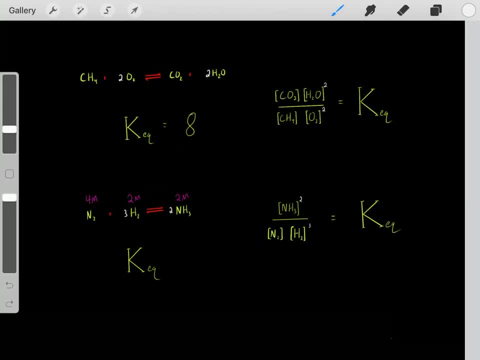 reactants, And then again we multiply them and put them to the respective powers. So again, we let it react. And once it reaches equilibrium, you take those equilibrium concentrations. It's those concentrations at equilibrium that you plug into this equation. So again, we let it reach. 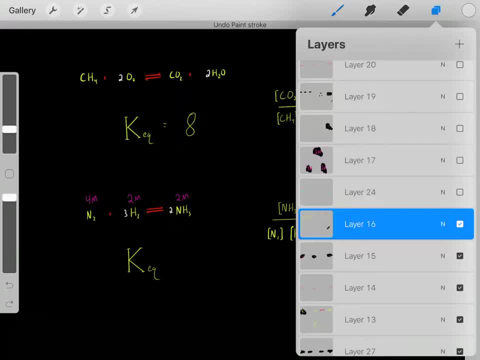 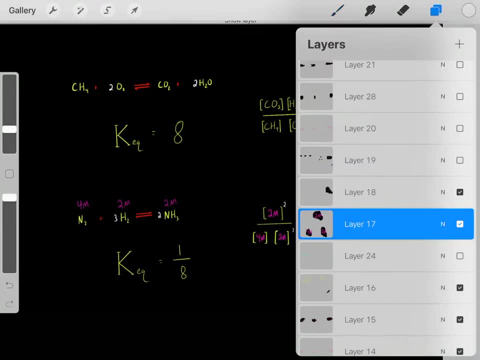 equilibrium. We get the equilibrium concentrations and we plug it into this equation. And if we did that, we'd plug in those values and just multiply it and just plug in. And if we did that we get a Keq of 0.125, which is 1 over 8.. So now we know this reaction has an. 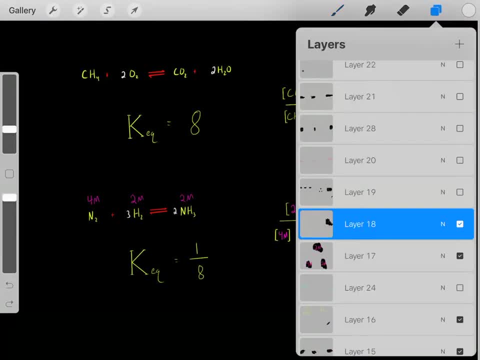 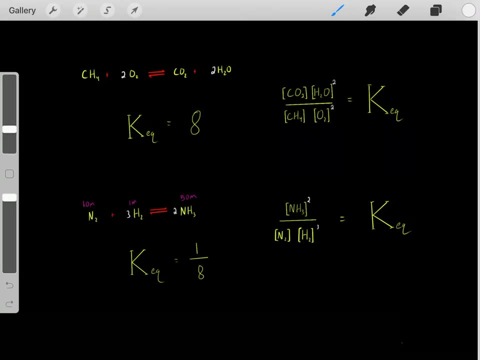 equilibrium constant of 1 over 8.. And again, remember, it doesn't matter what the initial concentrations were. Again, we could have any arbitrary initial concentrations. We'd let it react, We'd let it react and we let it reach equilibrium. Then we have equilibrium concentrations. 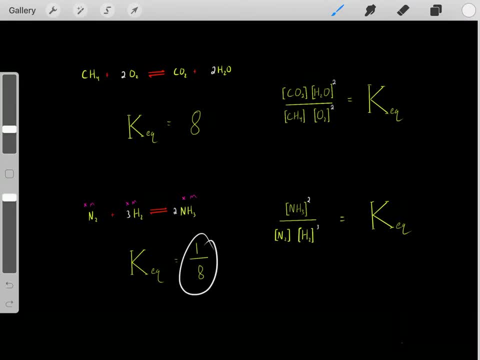 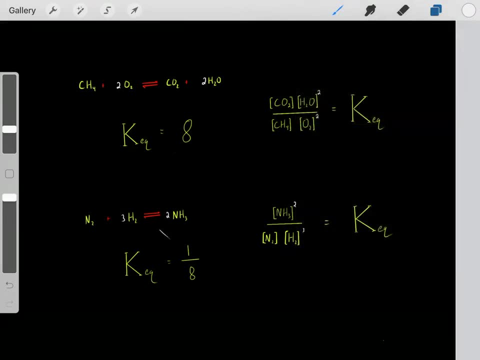 that we plug into this equation and it will always equal 1 over 8.. It's the equilibrium constant of the reaction. It's a constant. So now we know what equilibrium constants are and we know how to find them, just using this simple equation, where we take the products over the reactants and again, 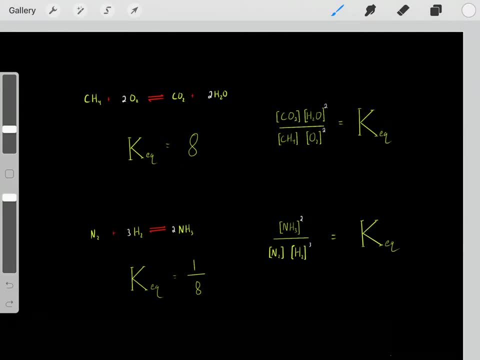 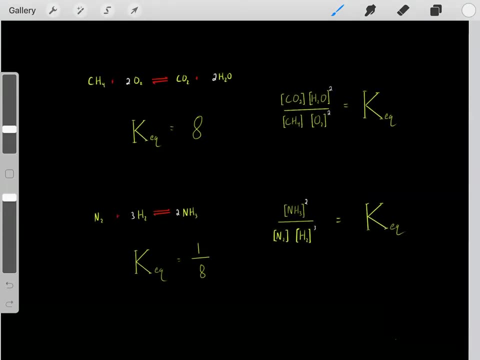 to their respective powers. But what do these equilibrium constants tell us? What does it mean that this reaction has an equilibrium constant of 8? What does that tell us? Well, really, what that tells us is when this reaction reacts and reaches equilibrium, there are a lot of products relative. 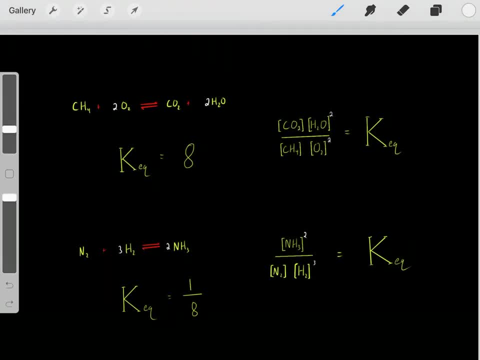 to reactants And that makes sense. It reacts to the equilibrium constant of the reactants. It reacts, It reaches equilibrium And then we take those concentrations at equilibrium and plug them into this equation. And if we have a lot of products, if we have a lot of products and very 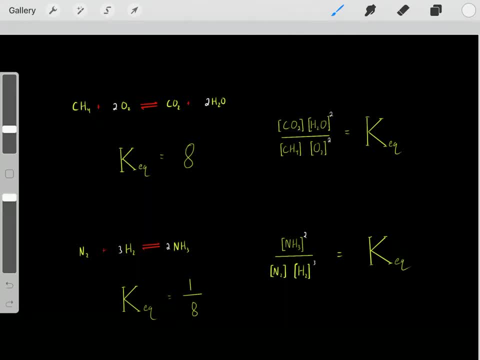 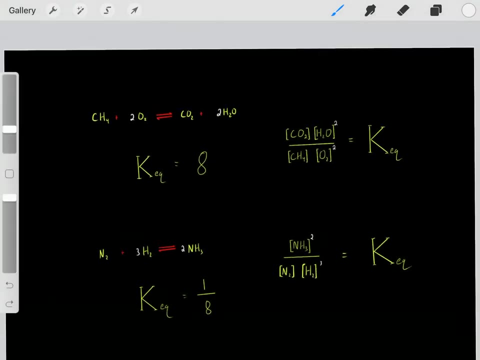 little reactants, we'll get a ratio of a number larger than 1.. So again, this Keq of 8 tells us that this ratio is 8. That means there's a lot of these products relative to reactants and therefore we have a ratio of larger than 1.. So if a Keq is larger than 1, that tells us when this reaction. 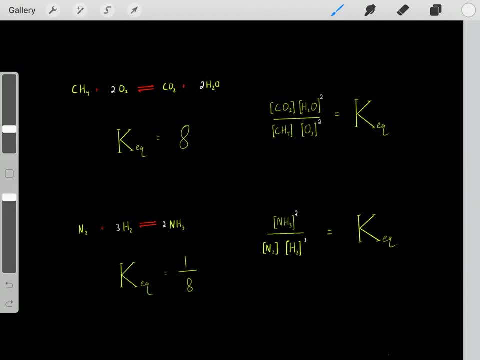 reaches equilibrium. there's a lot of products relative to reactants, And what does it mean if this reaction has a Keq of 1 over 8?? Well, that means this reaction reaches equilibrium. We plug in those equilibrium concentrations and we have relatively more reactants than products. And 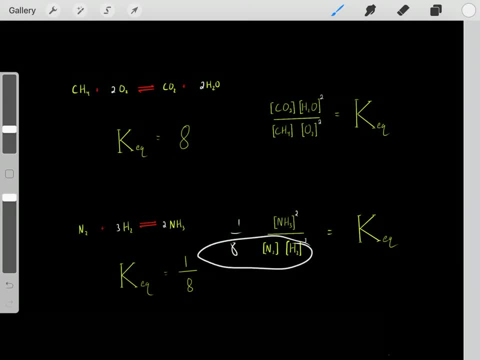 that's why we have a ratio of 1 over 8, because we have relatively more reactants than products. So that tells us that this reaction, once we reach equilibrium, there are more reactants relative to products And that's why we have a Keq of less than 8.. 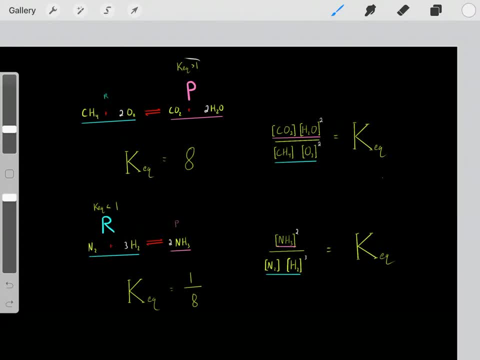 So the rule of thumb is: if a reaction has a Keq larger than 1, this ratio will be larger than 1 and we'll have more products relative to reactants. So this reaction at equilibrium, there are a lot of products relative to reactants. If we have a Keq that's less than 1, that means at equilibrium. 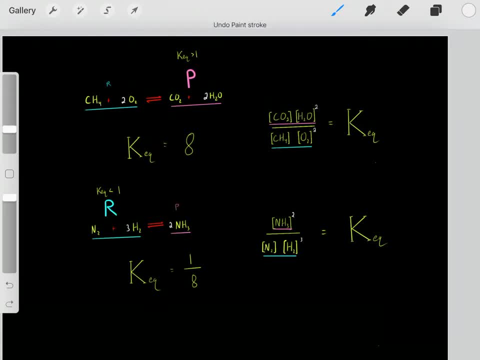 there's more reactants relative to products. We let this reaction react. It doesn't matter what the initial concentrations were. We let it react. It reaches equilibrium where there's more reactants relative to products, And that's why, when we plug it in, we got a Keq of less than 8.. And that's why 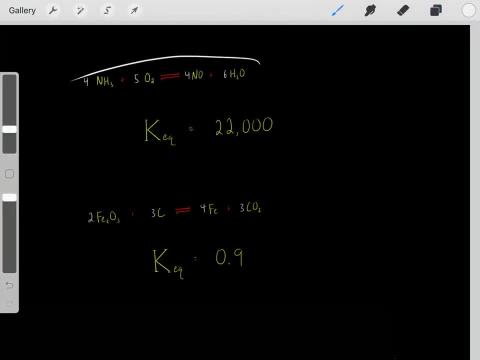 less than 1.. We got 1 over 8.. And just some examples. Let's say this reaction happens to have a Keq of 22,000.. Believe it or not, that's not absurd. You'll have reactions that have these. 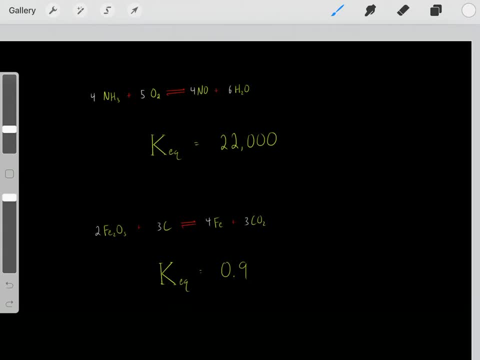 huge Keqs. But what does it mean if this reaction has a Keq of 22,000? That means we let this reaction react and at equilibrium there's a lot of products and very little reactants, And that's why we get this huge ratio And it's a little more complex, because we multiply them and then they go. 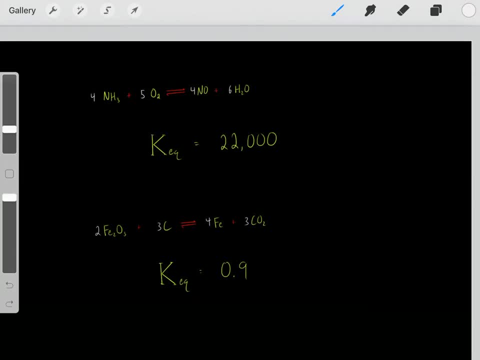 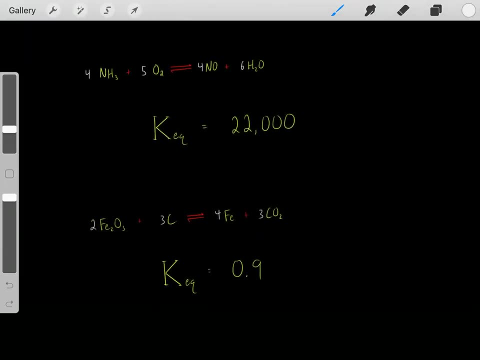 to these respective powers. But generally speaking, a Keq larger than 1, that means at equilibrium, a lot of products, very little reactants. This reaction, let's say, had a Keq of 0.9.. What does that mean? That means at equilibrium.